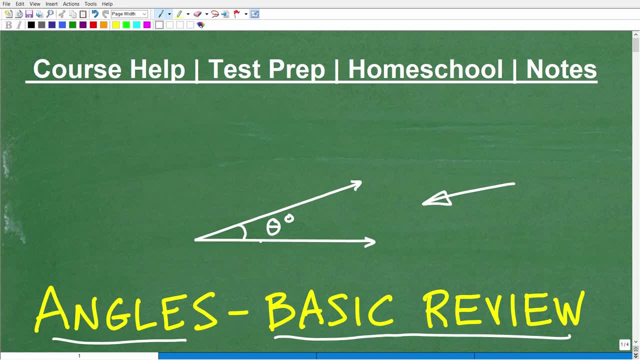 it doesn't have to be that way. I've been teaching math for decades And one thing that I really kind of learned along all those years of teaching math is that all students can really do very well in math One. of course you're going to have to have the desire to. 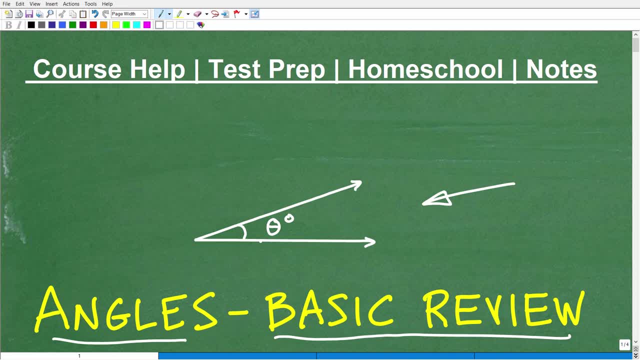 learn math, But two. what you need is excellent instruction, very clear and understandable instruction. You need someone to explain things to you. that's not like a textbook. Okay, and that's how I teach math. I really break things down and superimpose them into a textbook. 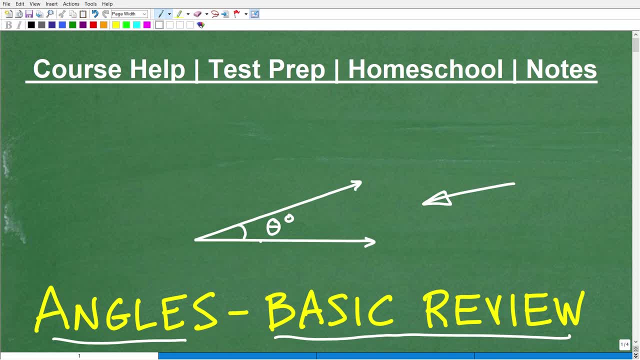 Super easy and understandable way so anyone and everyone can learn this stuff. So if you're at the middle school, high school or even college level in terms of mathematics, I can definitely help you out. Now, if you're preparing for some kind of sort of test that has a math section on, 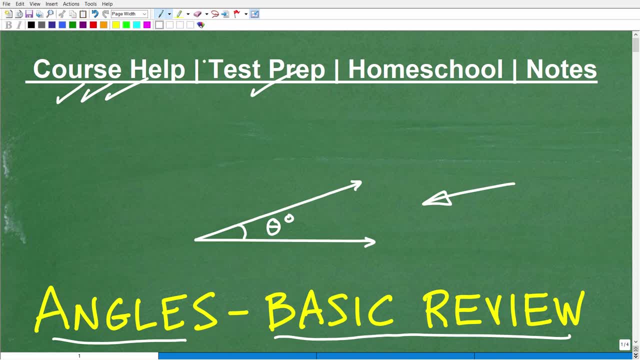 it. I'm talking about things like the GED, SAT, ACT, GRE, GMAT, ASVAB, ACCUPLACE or CLEP exam, maybe a teacher certification exam. I can help you prepare and pass those exams If you homeschool. 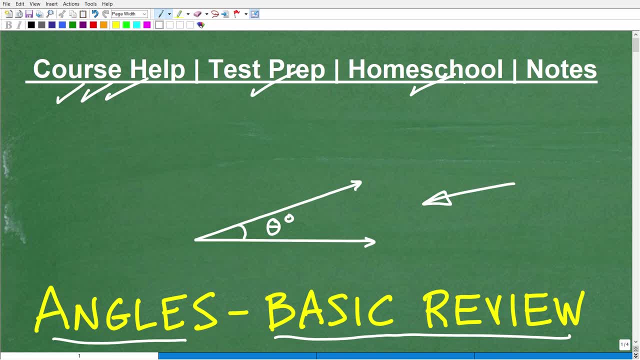 we were just voted number one for middle and high school mathematics in homeschool from your national publication. Please check out my homeschool math courses. You'll be happy that you did, And if you don't have any math notes, I'm going to leave links to my math notes in the 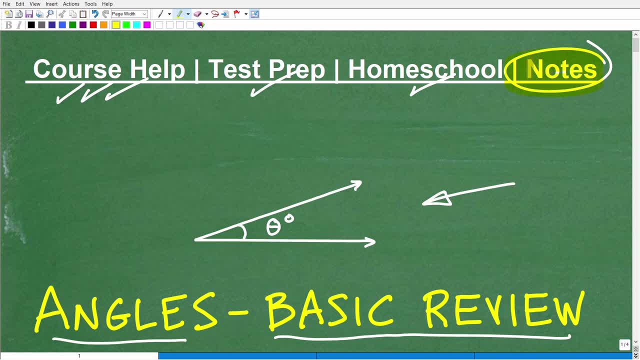 description of this video as well. But if you want to have excellent grades in mathematics, you've got to learn how to take great math notes. Okay, so let's get into angles Again. for the most part, everyone says: oh yeah, if I said what is this, you would say this is an angle. 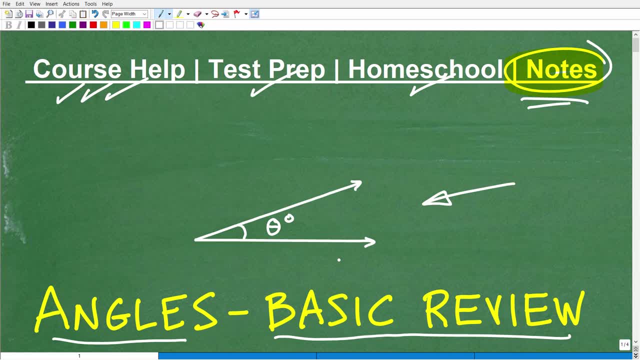 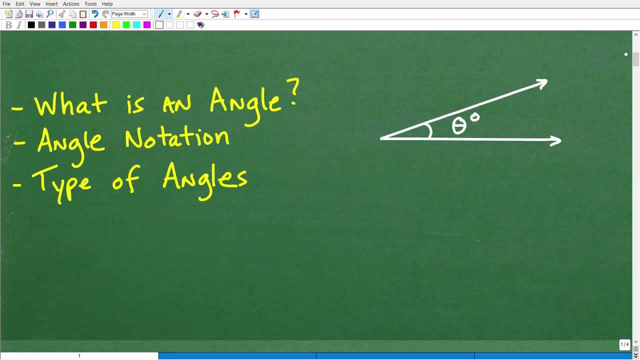 Okay. so again, most of us would recognize that, You know, if we saw one. but what is an angle? So let's get into this right now. So what is an angle? Well, basically, an angle is made up of two parts here. Okay, this thing right here. 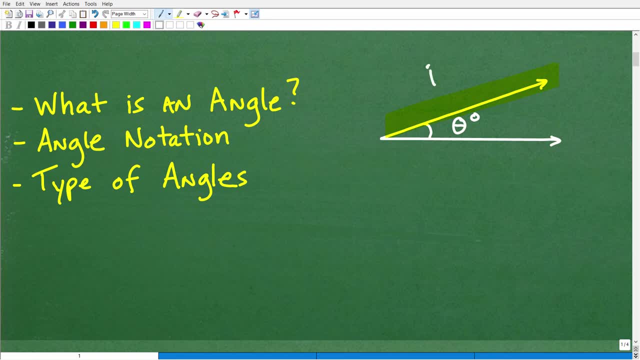 is a what we call a ray Okay on R A Y. So we have a ray right here and a ray has a starting point or an endpoint, Okay, and then it goes out in one direction, infinitely. Okay. so this is a ray right here And then this is another ray right there. So an angle has two rays. 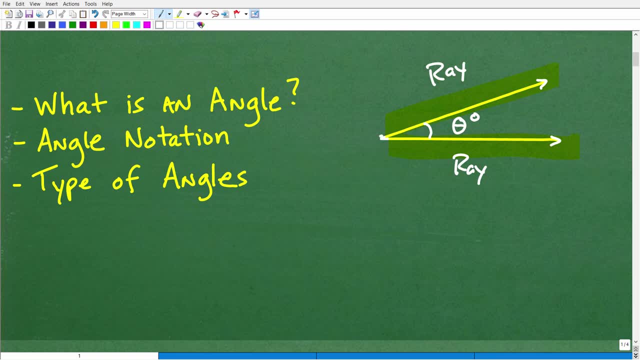 but they're kind of emanating or they're starting from the same start point, right there, Okay, and with a particular angle, or any angle that is. this point is called a vertex, Okay, so vertex is our starting point for two separate rays that emanate out from that point, which we call the. 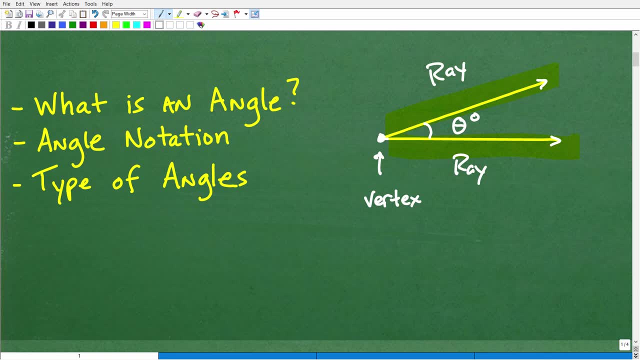 vertex. Okay, So this shape, this right here, is basically an angle. Okay, so it's made up of two rays and a vertex, All right. so hopefully you kind of remember that And I'm going to kind of just erase this so we can kind of stay on this. Now. again, this is just a basic review. 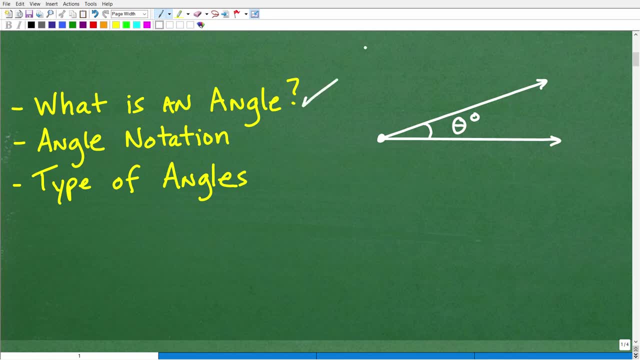 kind of just an informal review of angles. Okay, so what is an angle? We kind of answer that question. Now let's talk about angle notation. So how do we define this angle? Well, there's a couple different ways. we can do it in geometry. So if I wanted to say what is this? 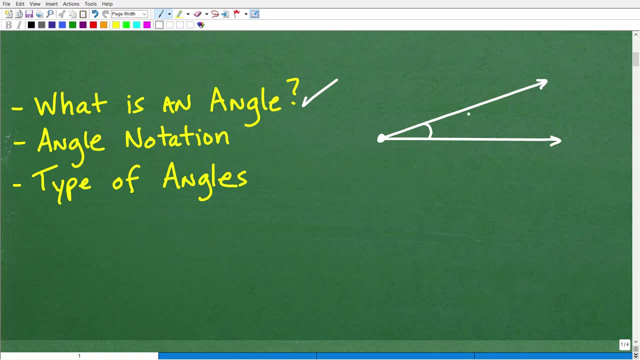 angle, right here describe it. I could call this, let's say, by a number. okay, let's say one. And now in geometry we use this little angle notation. So I could say: this is angle one, angle one, just like that. Okay, Maybe I can use a another variable like this: x. I can say angle x, That's. 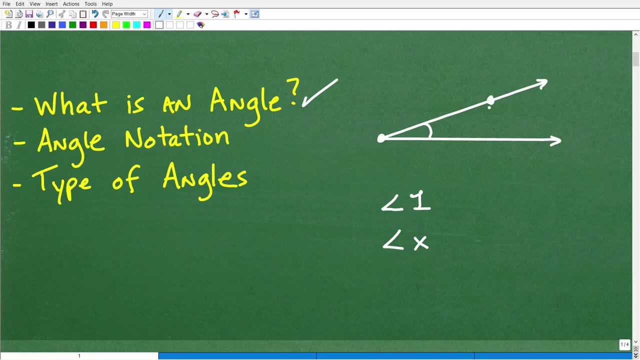 it. So another thing that's pretty common is if we have points that are on the rays. so let's say this is point A and then point B is our vertex and then point C is on this other ray. I could call this angle ABC. Now, when you're doing this, you have to go in actual order. So if I'm starting, 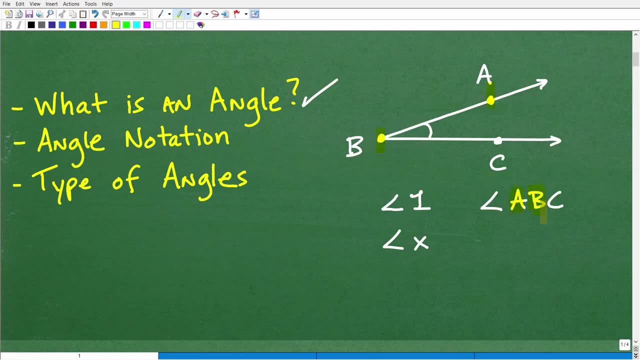 with A, I got to do B. next it's in the middle, And then, of course, we end with C, right here. Okay, Now, when you do use this type of notation to express an angle, this middle letter is always. 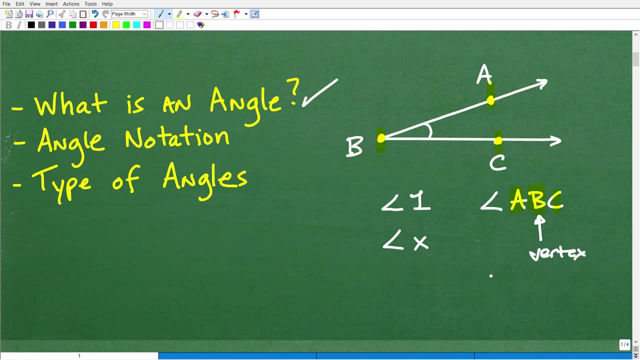 the vertex. Okay. Now, another way we could have done this: we could call this angle CBA. Okay So, but again, notice that the B, that middle letter, is the vertex. Okay, so that right there. So these are other points. So if you see points that are on the rays and you have the vertex, this is pretty. 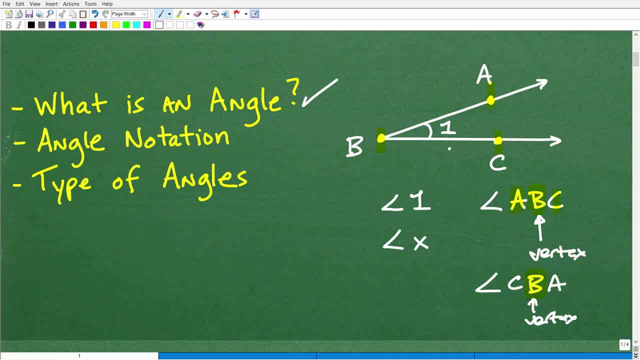 common. So we can express this angle with this little notation. But again, notice, we have this little angle notation, this angle little angle symbol. okay, in front of these different things. So this is very, very common, common ways to express angles. Now let's give this angle a. 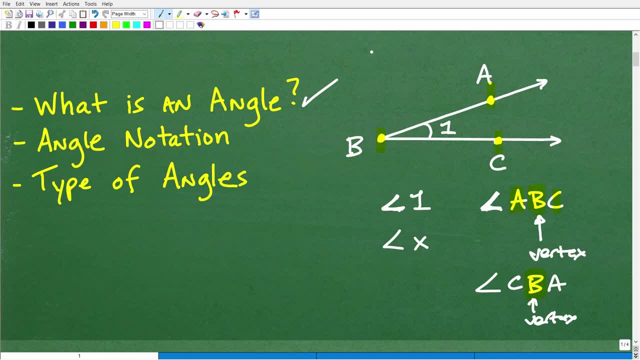 measure. So how do we measure angles? Well, there's basically two ways we measure angles. One is in degrees, Another one is in degrees And the other one is in degrees, So we have two ones called radians. I'm not going to really talk about radians right now. The most common way that 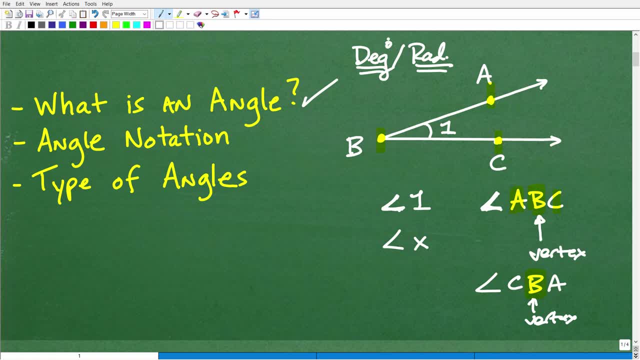 most people are used to seeing angles is with degrees. So degrees, let's just quickly review. If you start right here, zero in a circle, you go all the way around. you do one full lap around that circle, you do 360 degrees. Okay, let me write that a little bit better. I'm getting a 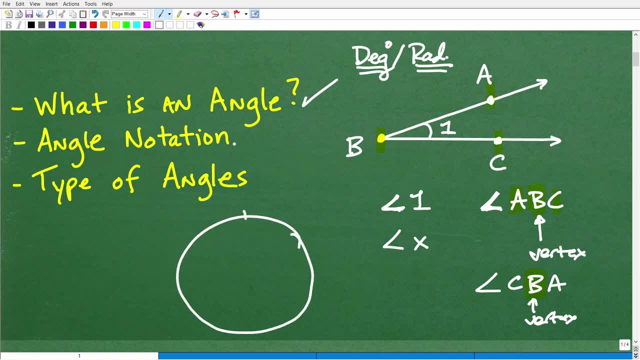 little sloppy here. I think it's because I'm trying to do everything in this one little window, But anyways, we go around, We start from zero and we end at the very top of the circle. we do one lap around the circle. 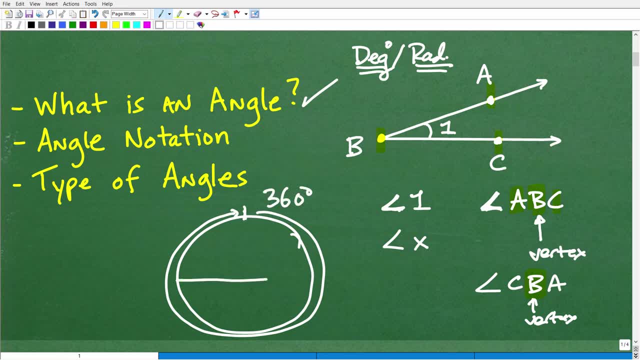 That's 360 degrees. Okay, So if I go halfway around a circle, which we call a semicircle, that's 180 degrees. If I go a quarter way around a circle, that's 90 degrees, And you can get the. 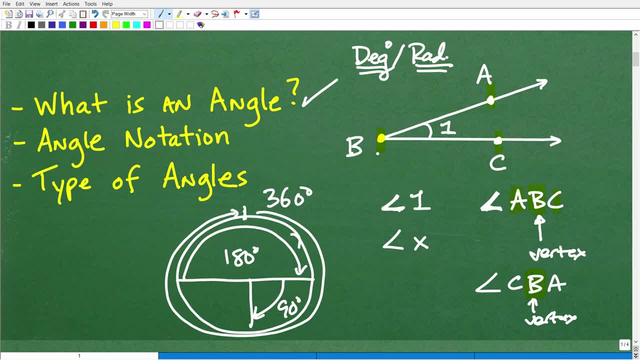 idea from there. So let me ask you right here how many degrees if you had to take a guess and estimate what this particular angle be? Okay. so let's just think about this for a second. One of the things in geometry they have to try to get pretty good at is estimating angle measurements. So looking at 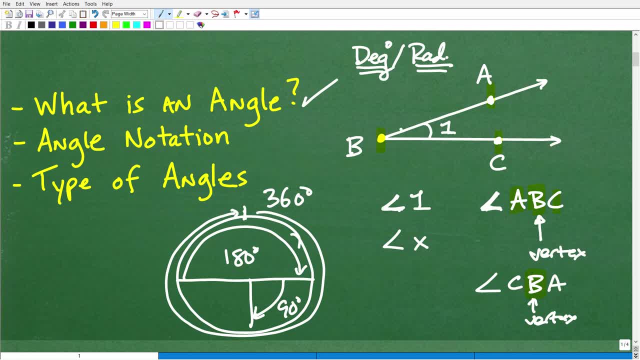 this, would you say. this is around 60 degrees. Okay, most of you, hopefully, said no, that's too big. This is probably around, like, say, 20 degrees or 20, less than 30 degrees. it looks to be maybe. 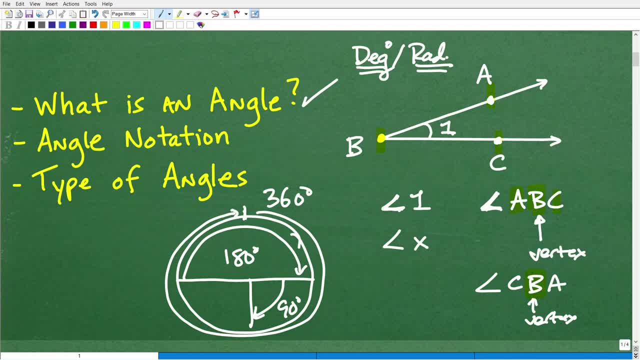 30,, 20 to 30 degrees. So we'll go ahead and let's just call this 30 degrees, Okay, So I'm going to go ahead and erase this And now let's say: use a different notation here to express: this angle right here actually has an angle measure of 30 degrees. So I can write it: 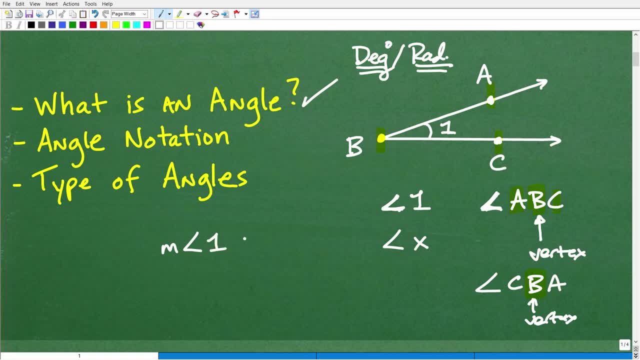 this way, the measure of angle one we'll use this notation is equal to 30 degrees. Okay, that's one way to do that. Sometimes you'll see it as congruent to 30 degrees like this. All right, typically you'll see it equal, or? 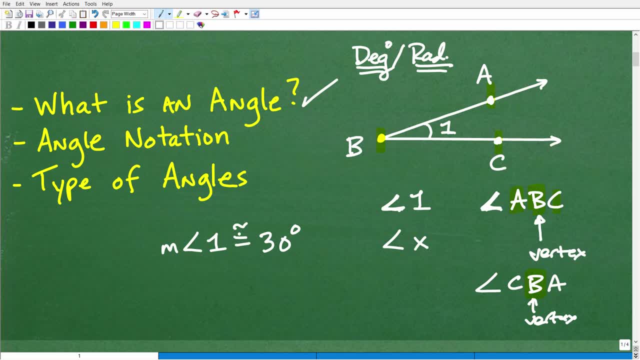 you'll see it as congruent to 30 degrees. So I'm going to go ahead and erase this. And now let's say you won't see this symbol. sometimes you'll see this symbol as well. it all depends on you know the textbooks and how people are teaching this. But when we're talking about 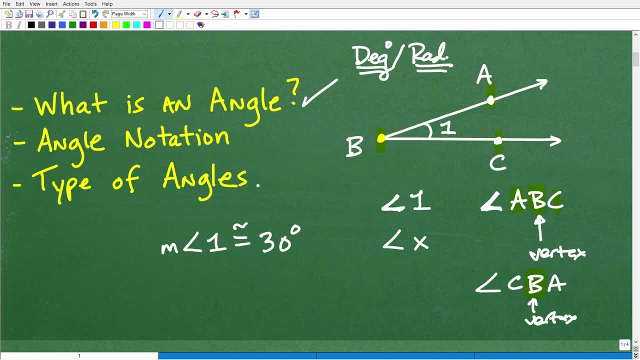 angle measurement or lengths and whatnot. you are talking about congruency. Sometimes you'll see this particular notation, Other times you'll see the equal sign, But basically, what you want to do is put this little M in front of the angle. very, very common way. 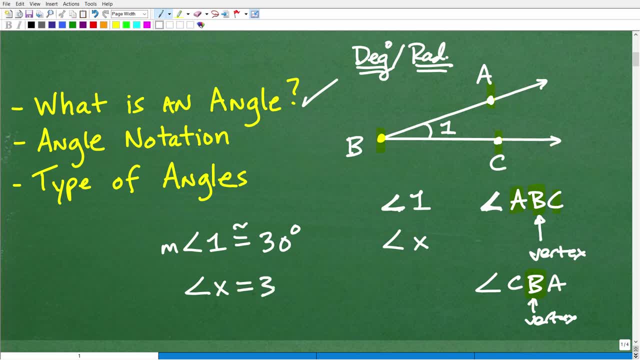 Sometimes you'll see it this way: like angle x is equal to 30 degrees, So if you see it in this particular way, stylistically, that's fine as well. Okay, Now let's go back and talk about this other way of writing angles. 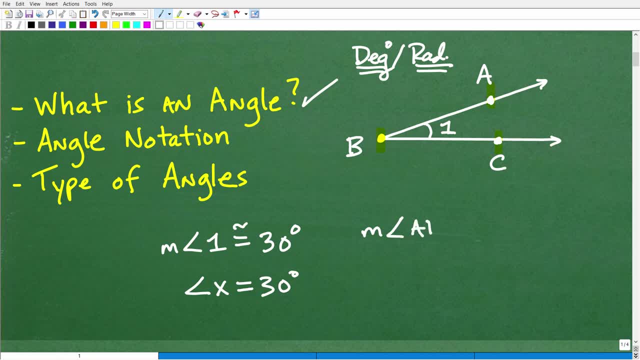 I could put all right: the measure of angle a, b, c is congruent to 30 degrees, or has an angle measure of 30 degrees, or the measure of angle a, b, c is equal to 30 degrees. Okay, 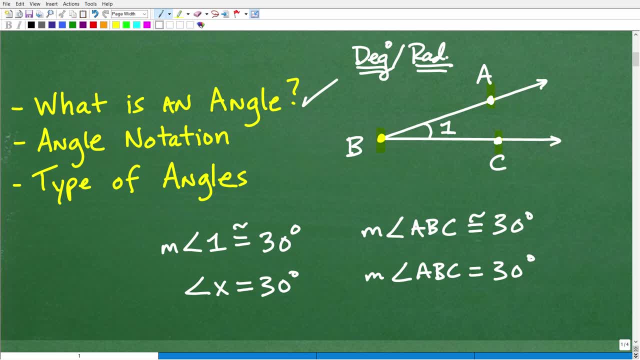 so pretty standard notation. And again, if this little M right there, that means the measure of that particular angle is this many degrees. Now again, I talked about this thing called radians. Let me just tell you very quickly when you go full lap: okay, we want to talk about radians. That is what we call 2 pi radians It. 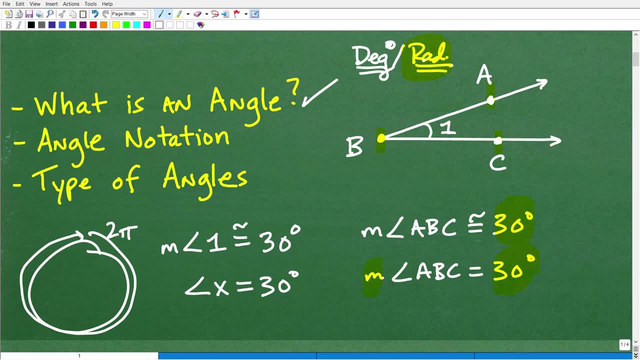 doesn't have a little degree symbol to it And you're going to study radians pretty heavy duty. when you get into trigonometry and you actually express angles as you proceed in more advanced mathematics, You might even find radians as a more common measure of angles, even beyond degrees. 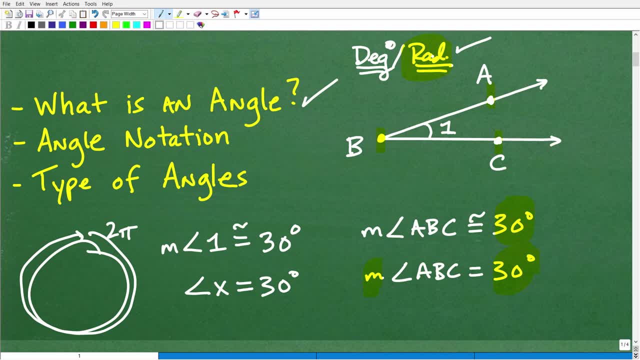 Okay, so just because I'm not really mentioning radians right now, as you study trigonometry and get into even more advanced mathematics, you're going to be very familiar with radians and you'll learn how to go from radians to degrees and degrees. 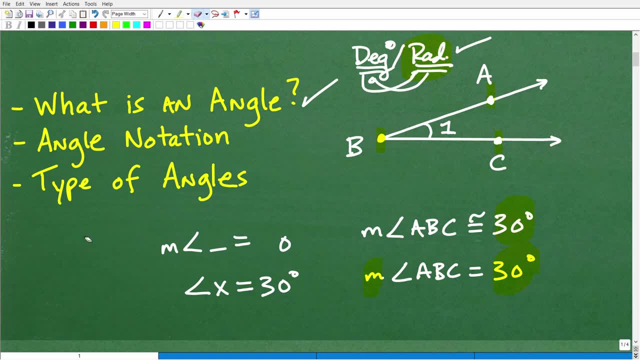 But right now we're kind of- this is kind of sticking to the basics about angle concepts, Okay. so, anyways, let's get into types of angles, All right. so we talked about what an angle is: two rays that emanate from that same vertex, that one point angle notation. We 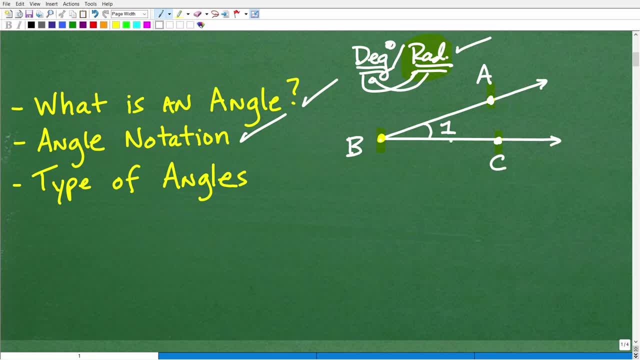 talked about various type of ways to express an angle and to specify an angle measure. Now let's talk about the types of angles. So the way I want to do it is this: I'm going to go this way, All right, and you'll see why I'm doing. 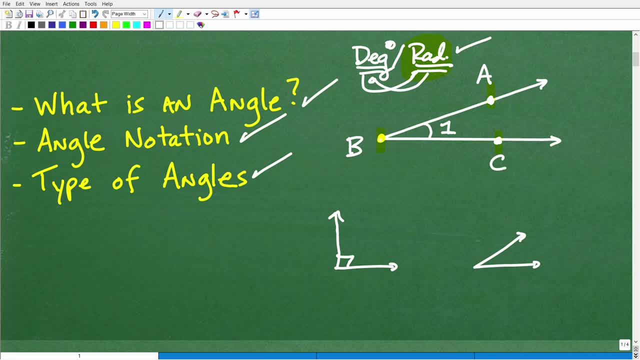 this in a second. Now I'll give you an opportunity to try to name these angles. Okay, the different types of angles. Okay, so let's start over here And let's play this game, All right? so these are basically the four different types of angles. So this type of angle starts with an A. Let's see if. 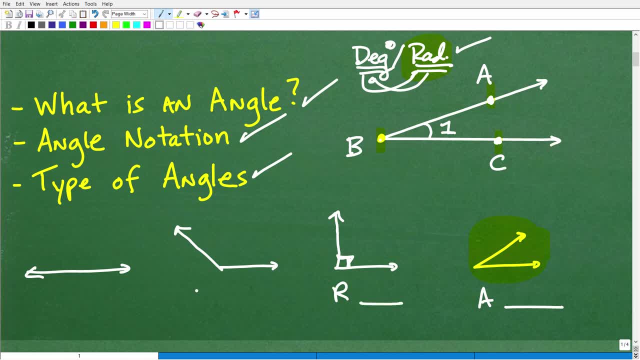 you can do this. This type of angle starts with an A, And then this type of angle starts with an A, This one starts with an R, This one starts with an O And this one starts with an S. Okay, so let's. 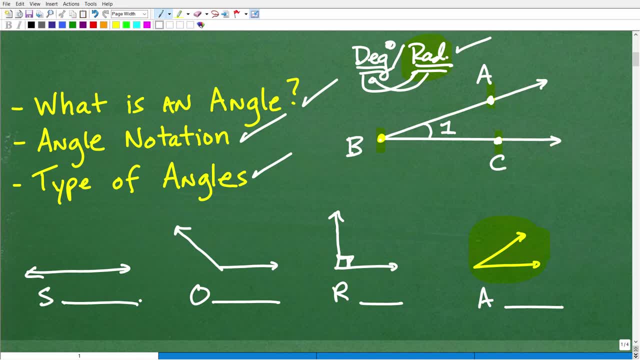 play this game here. Okay, so these are the different types of angles. So what type of angle is this? Well, if you said acute, all right, this is an acute angle, you would be correct. Okay, so what is an acute angle? Well, we're looking at it. You're like, well, acute, And just think about. 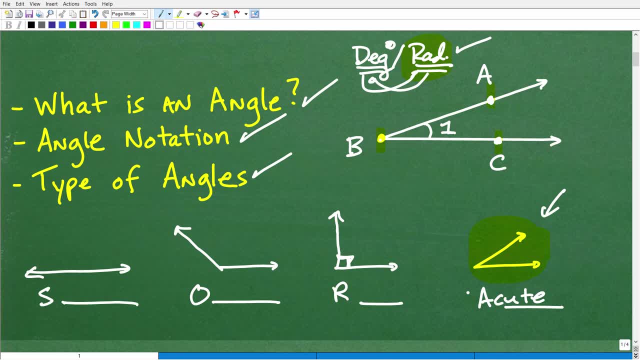 this word acute. If you go to the doctor and the doctor says, do you have acute pain? They're like pushing on your belly and stuff- You're like ouch, that's. you know that hurts That word acute. it's also another kind of it's synonymous with the word sharp. Okay, so any angle. 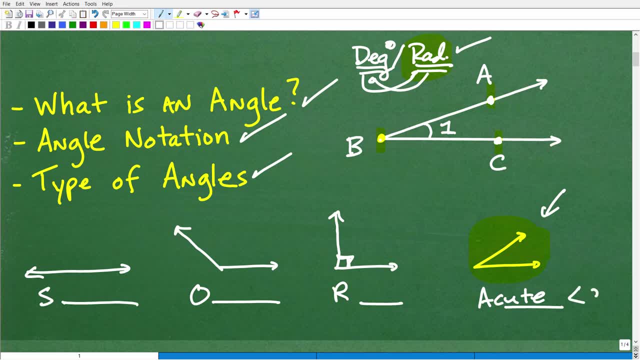 that's less than 90 degrees. okay, less than 90 degrees is considered an acute angle, Okay, but you kind of think of that word acute as being like sharp, Okay. so it's kind of interesting how some of these terms are used, you know, outside of you know vocabulary terms. 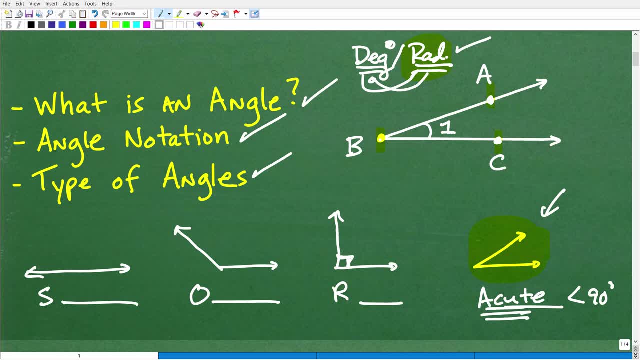 Whether it's an acute angle or acute pain. All right, we're talking about something that's sharp, Okay. so acute angles: less than 90 degrees: Okay. so that brings us to our next angle here. And notice, I have a nice little symbol here, the little box in the corner. This is a? what type of? 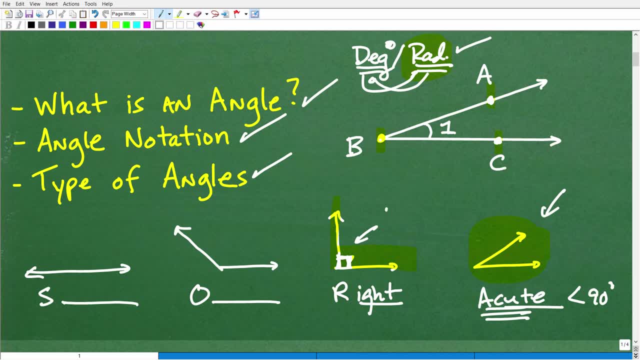 angle. This would be a right angle, And a right angle has 90 degrees. It's exactly a 90 degree angle, And that's like the corner of a square or a rectangle. That's what a 90 degree angle is. So we have a right angle, Okay, which is 90 degrees, And it's 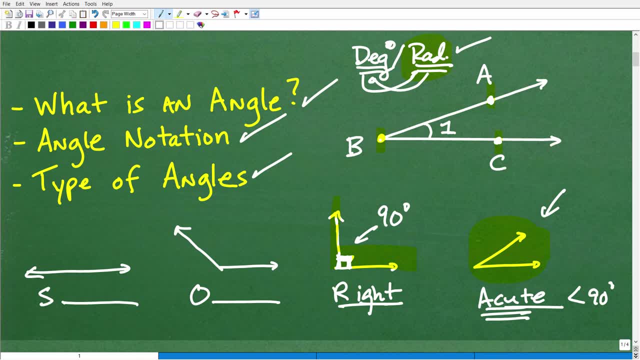 indicated by this little notation like this: So we have acute, we have right, and now we have this type of angle. So this time, type of angle is what? Well, it's greater than 90 degrees And we call this an obtuse angle. Okay, obtuse, Now again that word obtuse, and I don't want to make anyone 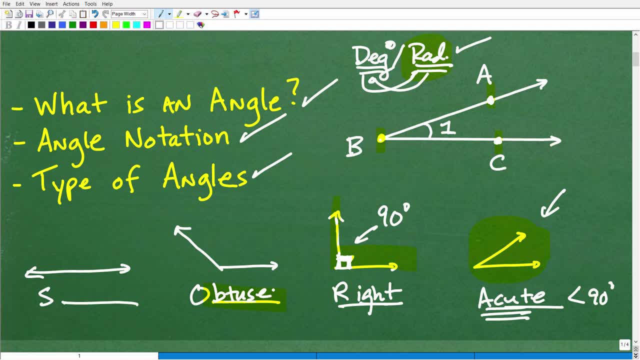 feel bad, but that's also an adjective that's used if you were saying that person's obtuse. that means they're kind of dull, all right, or maybe not, you know, as bright as some people might think They're like, well, that's obtuse or it doesn't. make you know it's not, it's the. 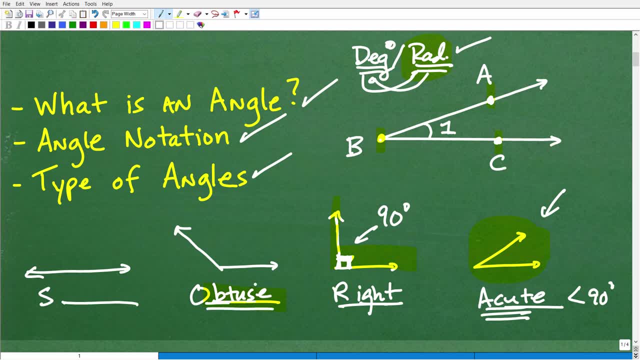 opposite of sharp. Okay, so just look up these definitions. you'll see various ways that the word obtuse and acute can be used. But obtuse angles are greater than 90 degrees. Okay, greater than 90 degrees. So actually we'll do it this way: Angles that are greater than 90 degrees. 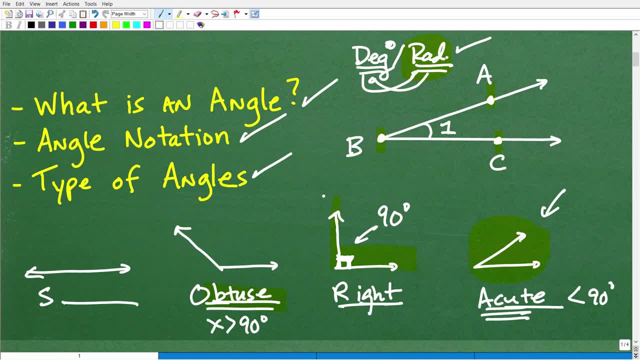 are obtuse. So less than 90 degrees acute, exactly 90 degrees right, greater than 90 degrees obtuse. And then we got this last one. Okay, so what is this one right here? Well, some of you're like saying: well, this doesn't even look like a, an angle. Okay, because I don't see two rays. 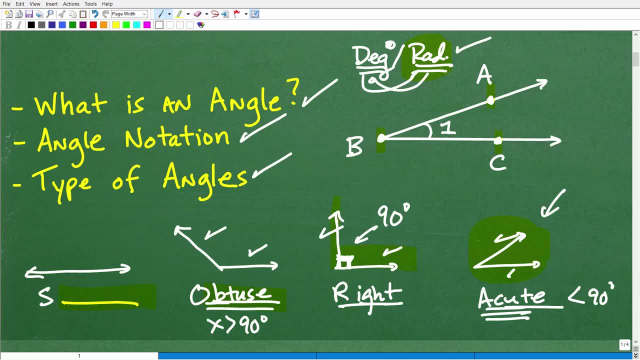 Here's a ray, here's a ray, there's a ray. there's a ray, here's a ray, here's a ray, a vertex, a vertex and a vertex. So all these look like angles, but this just looks like a straight line. 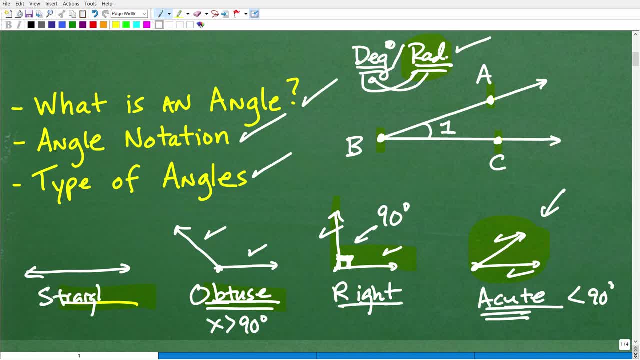 right. Well, actually this is called a straight angle, Okay, so there's the vertex right here, there's one ray going out that way, there's another ray going out this way, And straight angles are actually exactly 180 degrees. Okay, so that is an angle in and of itself. So it's an